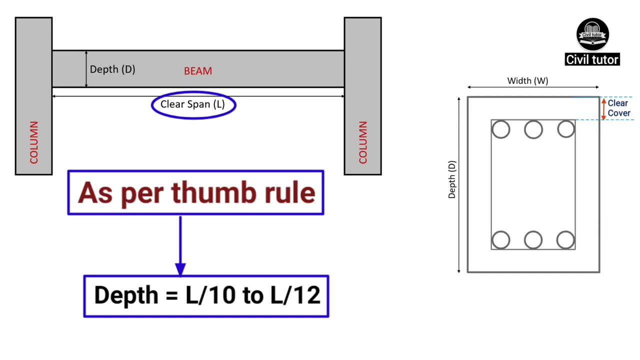 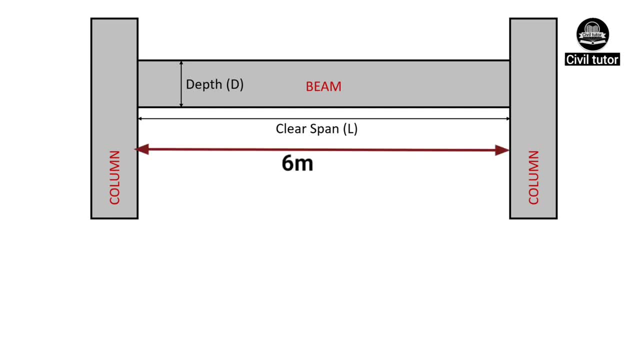 L is the clear span of the beam. By the term clear span we mean the column inner to inner distance. For illustration, let's consider a beam having a clear span of 6 m. The depth of this beam will be given by depth equal to L upon 10 or L upon 12,, ie 6000 upon. 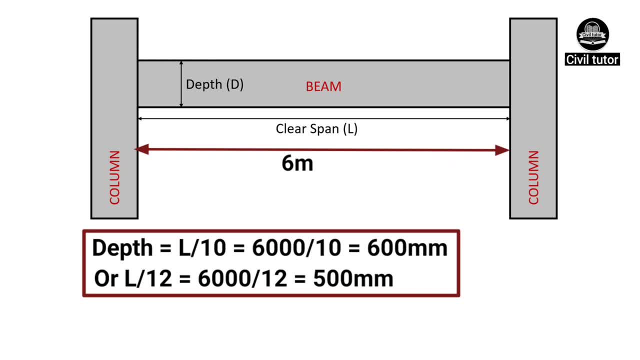 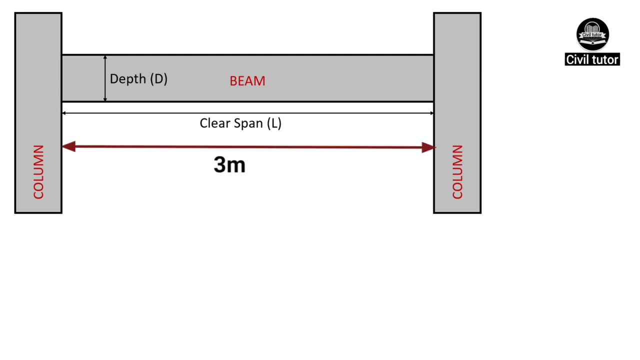 10 or 6000 upon 12,, which will be same: 600mm to 500mm. Hence, we can choose any depth between 500mm to 600mm for a 6m clear span. Let's take another example of a beam having a clear span of 3m. Its depth will be given. 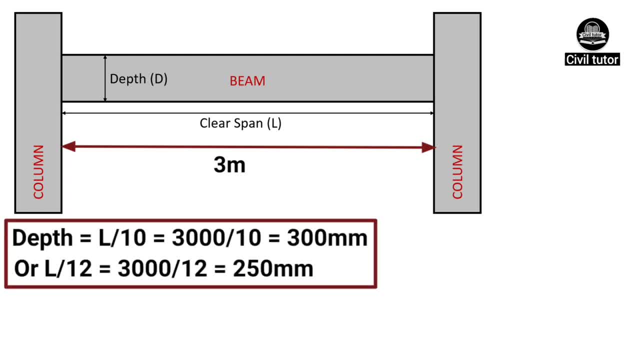 by Depth, equal to L by 10, which is 3000 upon 10, equal to 300mm, or L by 12, which is equal to 3000mm upon 12, which will be equal to 250mm. For calculating the width, the ratio of width. 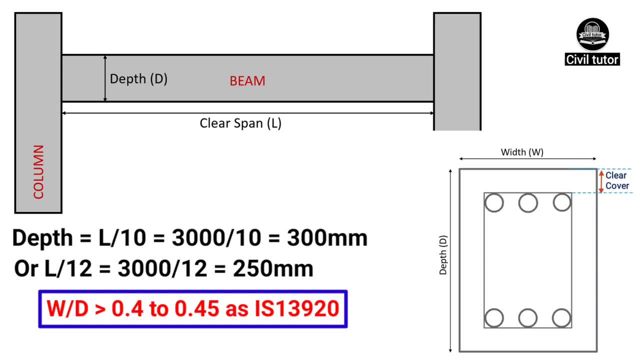 to depth should be greater than 0.4 to 0.45 as per IS 13920, ie, W by D should be greater than 0.4 to 0.45, where W is the width of beam and D is the depth of beam. It should be noted. 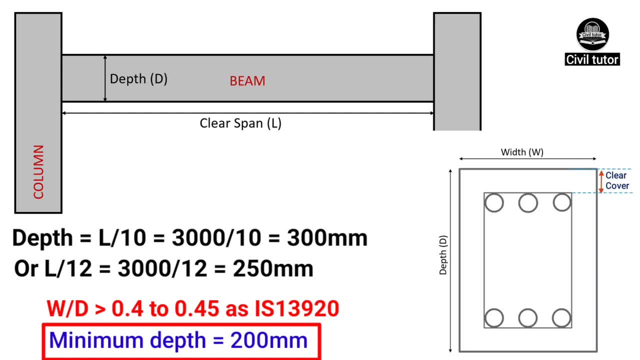 that the minimum depth should be kept as 200mm. For illustration, if we have a beam with a depth of 0.4 to 0.45,, the minimum depth should be kept as 200mm. For illustration, if we have a beam with a depth of 0.4 to 0.45,, the 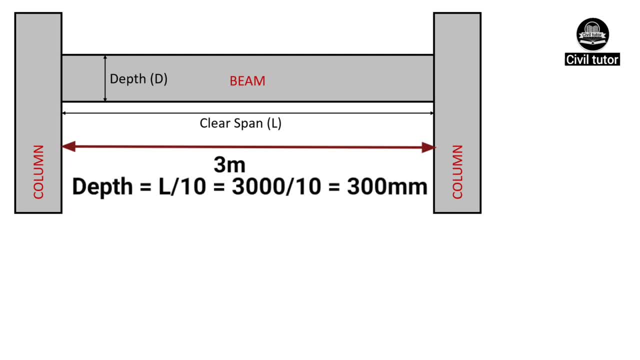 maximum depth should be kept as 20 mm, For錯. The ratio of W by D will be equal to 200 upon 300, which will be equal to 0.66, which is greater than 0.4.. Hence, it would be safe to go with 200 mm width for this beam. 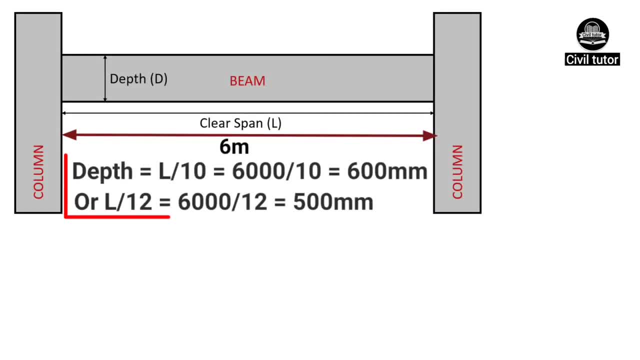 Let's take another example of a 6 metre span. The depth will be given by 6000 upon 10, which 600 mm, or 6000 upon 12, which will be equal to 500 mm. let's choose 550 mm as its depth. 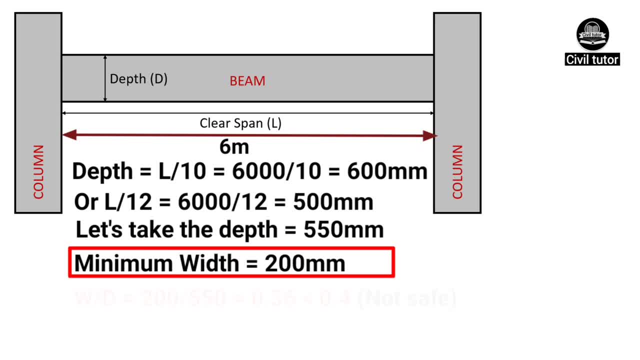 now let's provide the minimum width equal to 200 mm. the ratio of w by d will be 200 upon 550, which will be equal to 0.36, which is less than 0.4. now let's increase the width to 250 mm.